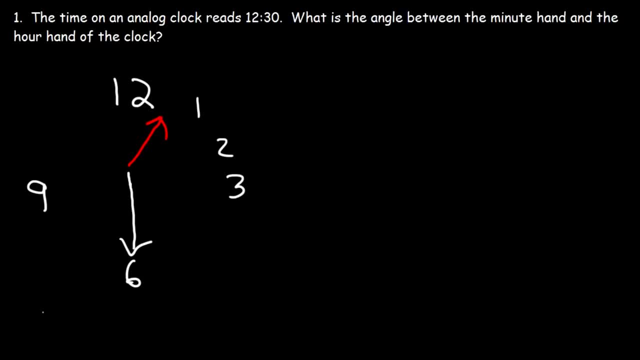 So that's 1230.. Our goal is to find your clock. What is the angle between those two hands? So how can we do so Now? first, it's helpful to know the measure of one hour, So let's focus on the 3.. 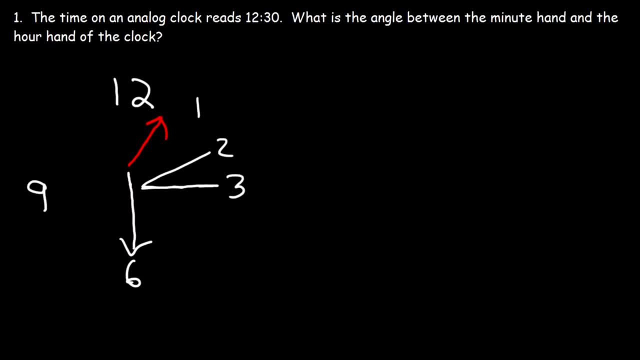 What's the angle between the 2 and the 3?? Notice that it takes 12 hours for the hour hand to make a complete revolution. So 12 hours correlates to 3.. So that's 360 degrees, because that's the entire circle. 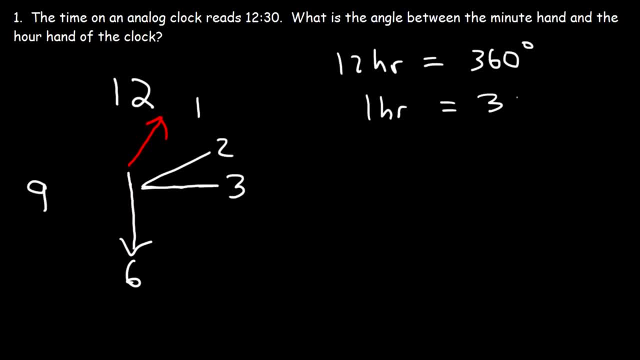 So one hour is going to be 360 divided by 12.. So every hour represents an angle of 30.. So therefore, from 1 o'clock to 6 o'clock, that's a time period of 5 hours. So if one hour represents 30 degrees, 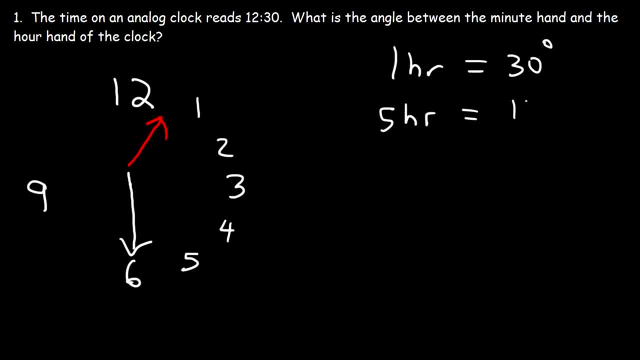 then 5 hours is 5 times 30, which is 150 degrees. So therefore, from 1 all the way to 6, that angle is 150 degrees. So now we need to find it, from this point to this point, this angle here. 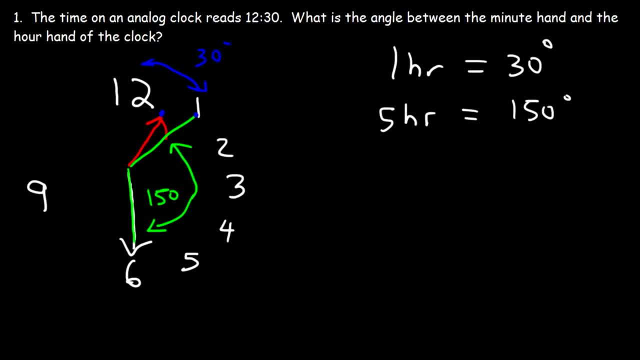 Now we know, from 12 to 1, it represents 30 degrees. So the red line is right between 12 and 1, because we're at 12.30, we're halfway between 12 and 1.. So if we're halfway we need to multiply 30 by half. 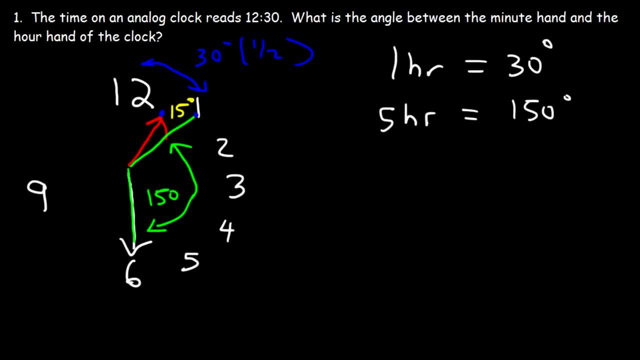 So therefore, the angle on the inside is 15 degrees, So we gotta add 150 and 15.. Therefore, the angle between the hour hand and the minute hand is 165, which is less than 180.. Because if the hour hand was at 12 and the minute hand was at 6,. 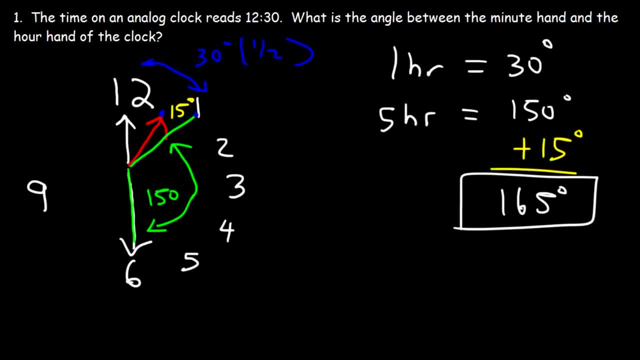 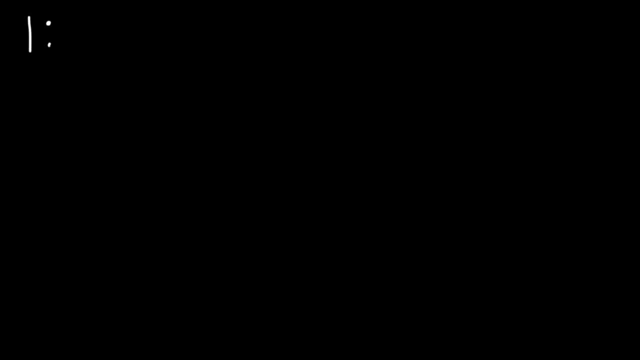 which is impossible. that would be a straight line, that would be 180, but it has to be less than 180. And this answer is reasonable. Here's another example: Convert the time 120 to degrees, That is, find the angle between the hour hand and the minute hand. 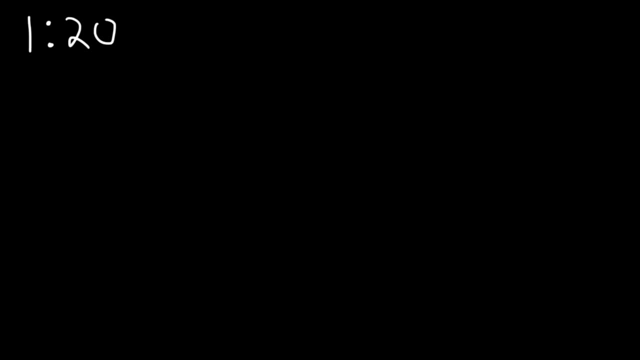 if the clock says 120.. So first let's draw a picture. Here's 12,. this is gonna be 3,, 6, and 9.. And then here's 1,, 2,, 4, and 5.. 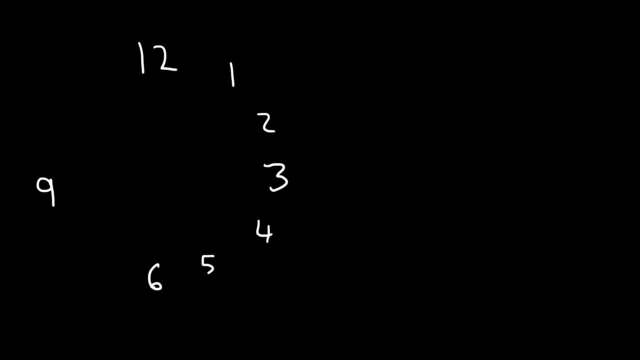 So if it's 120, that means the hour hand is between 1 and 2.. The minute hand has to be at 4.. So I'm gonna use blue to represent the minute hand, Which is the long one, And red to represent the hour hand. 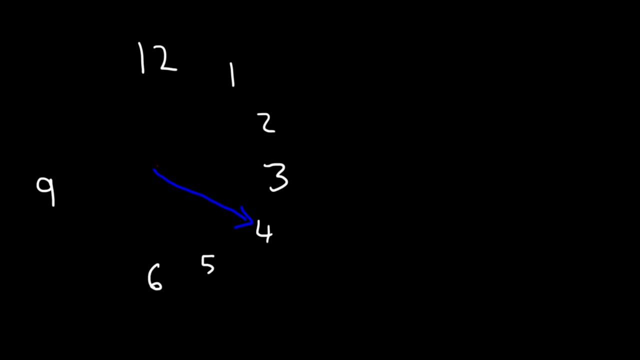 Now, if the hour hand is between 1 and 2, where exactly is it So focus on the minute hand, which is at 20.. 20 divided by 60 is a third. So what this means is that the hour hand is one third away from. 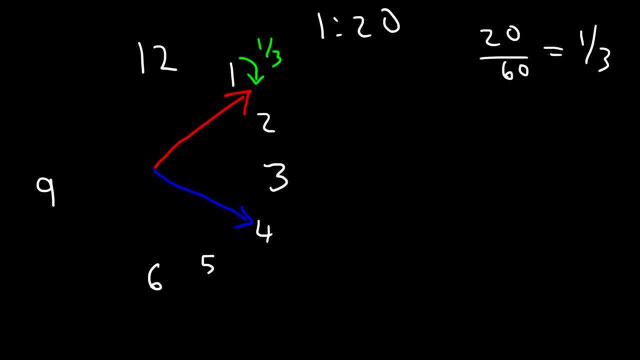 the one o'clock hour or the value of 1.. And it's two thirds away from the second hour or from 2.. So that's why you want to take whatever your minute value is and divide it by 60. So you can get. 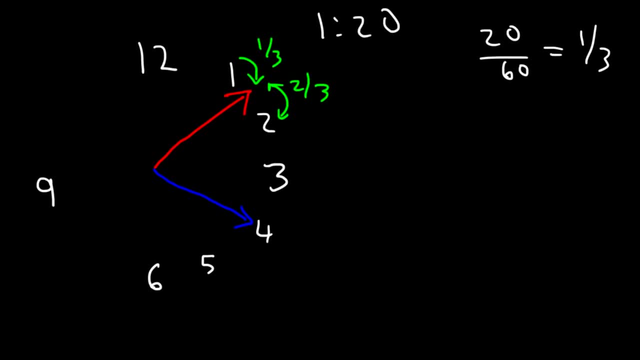 the fraction of how far it is from one of the hours And to find the distance from the other one. it's gonna be 1 minus the original fraction. So 1 minus one third will give you two thirds. So now with this information, 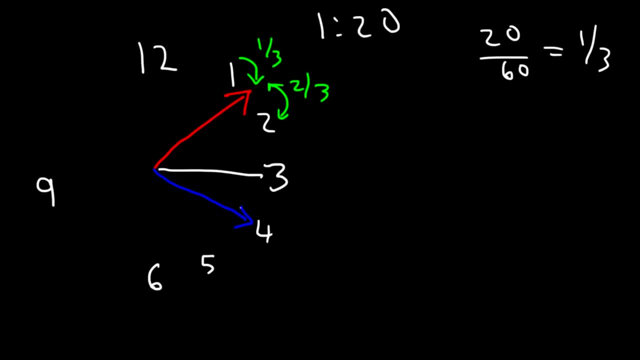 we can find everything we need. So keep in mind the angle between one hour is always 30 degrees. It's 360 divided by 12.. So between 3 and 4 is 30 degrees and between 2 and 3 is 30.. 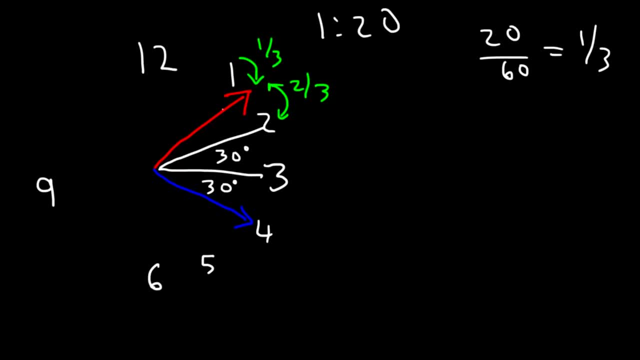 Now here is where it gets interesting. So this is when you want to use this fraction. This angle is two thirds of an hour. That's the missing 40 minutes. So the angle for one hour is always gonna be 30.. 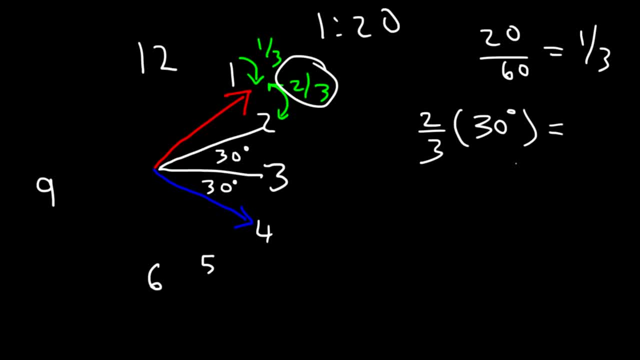 That's not gonna change. We gotta find two thirds of 30.. 30 divided by 3 is 10, times 2 is 20.. So therefore, this angle is 20.. Now all you need to do is add up these three angles. 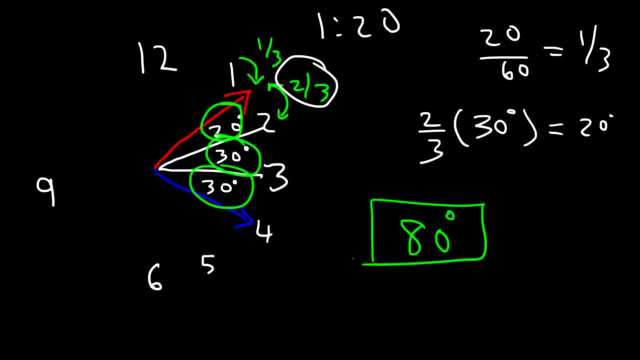 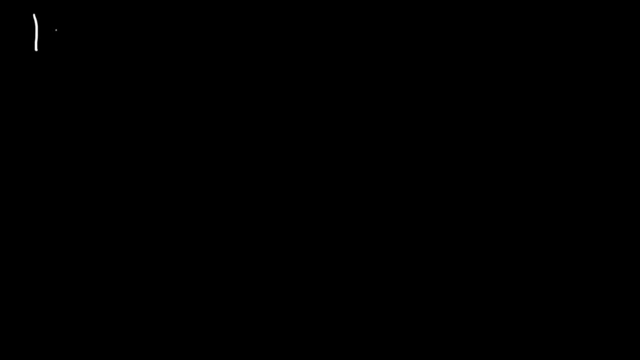 20 plus 30 plus 30 is equal to 80.. So that is the angle between the hour hand and the minute hand, And that's how you do it. So now it's your turn. Try this example: The time on an analog clock. 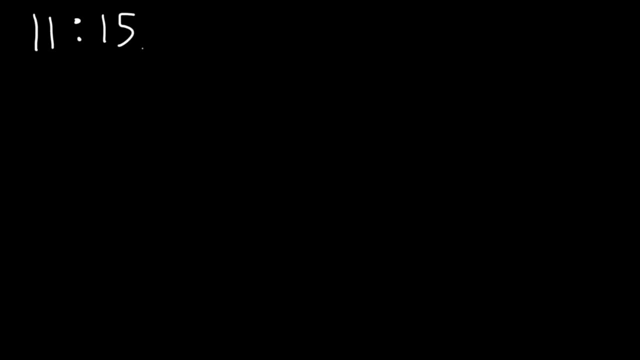 is 1115.. Go ahead and find the angle between the hour hand and the minute hand. So feel free to pause the video and work out this problem Now. let's always begin with a picture. So this is 12,, 3,, 6,. 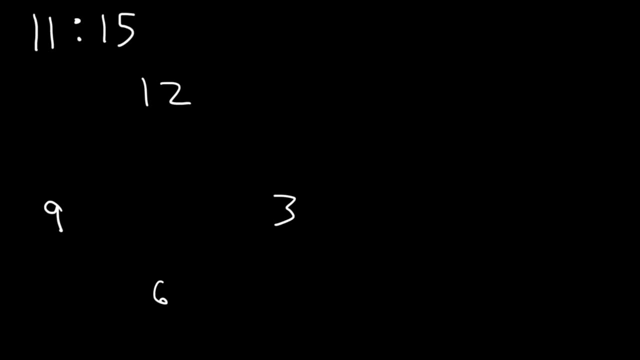 and 9.. The minute hand is at 3, because it represents 15.. 3 is for 15,, 6 is 30,, 9 is 45,, 12 is well 0.. So every increment of 5. 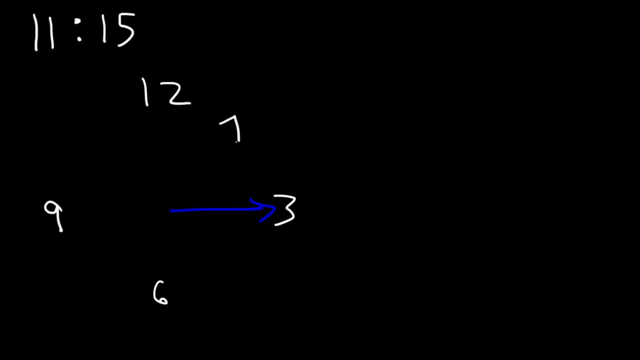 is for each number. So, for example, let's put down the other numbers. So let's say, if it was 1105.. The minute hand will be at 5.. 1110, it will be at 2.. 15 is for 3,. 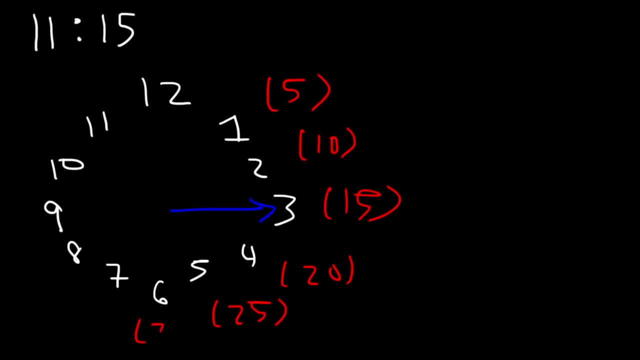 20 is 4,, 25 is for 5,, 30 is for 6,, 35 is for 7, and so forth. 55 is for 11.. This is 50,, 45,, 40, and then back to 0.. 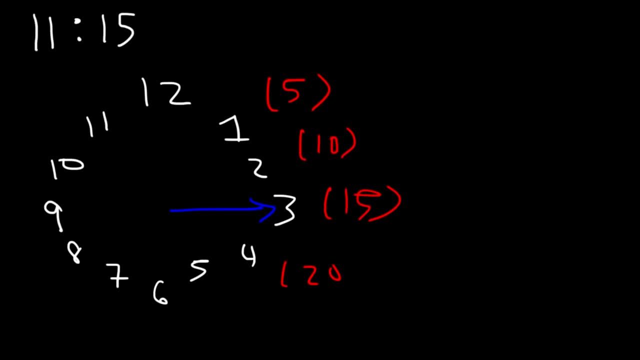 So, just in case you were wondering, those are the numbers that you need to know. So the 15 points to 3.. Now, where is the hour hand? We know that the hour hand is between 11 and 12.. But it's closer to 11.. 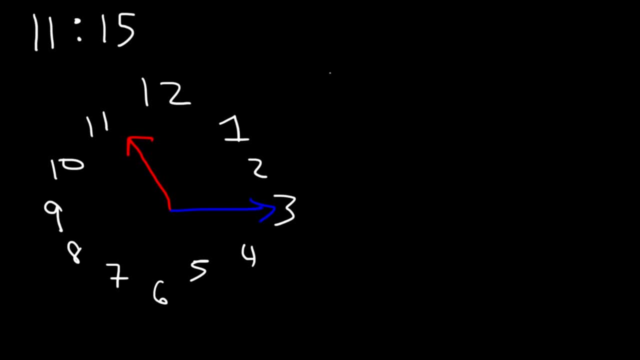 What we need is the fraction. So take 15, the value of the minutes, and divide it by 60.. 15 over 60 reduces to 1 fourth. So therefore the hour hand is 1 fourth its way from the 11th hour. 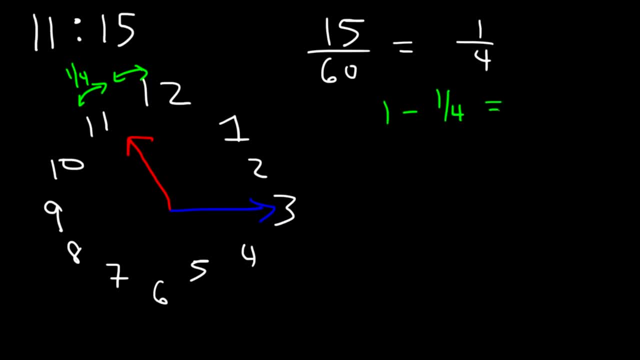 Which means that if we subtract 1 by a fourth, it's 4 over 4 minus 1 over 4.. 4 minus 1 is 3, so 3 fourths is between the hour hand and 12.. So it's 3 fourths. 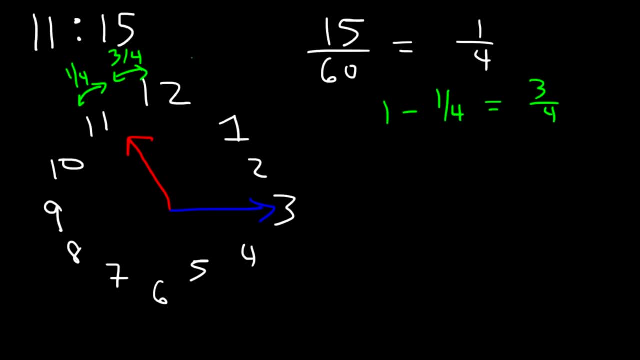 it's 1 fourth of the way going from 11 to 12.. It has 3 fourths left to get to 11 and 12.. So basically, it's 25% of the way between 11 and 12.. Now that we have that, 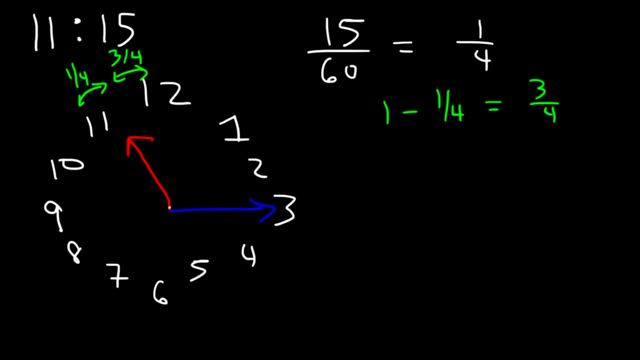 let's go ahead and calculate the angle. So every hour represents 30 degrees. Now the angle between the hour hand and 12 is going to be 3 fourths of 30. So what is 3 fourths of 30?? 30 divided by 4 is: 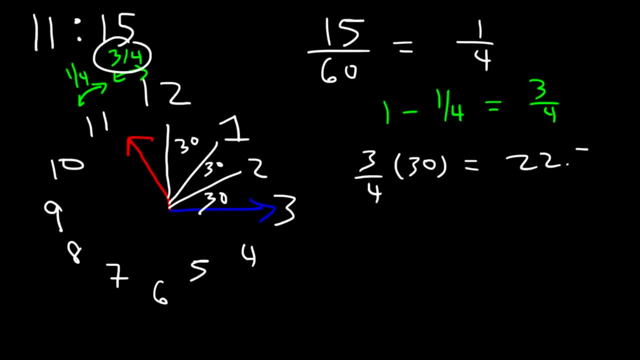 7.5.. 7.5 times 3 is 22.5.. So that's the missing angle. So if we add 30 three times, we get 90. So we get to add 90 plus 22.5.. 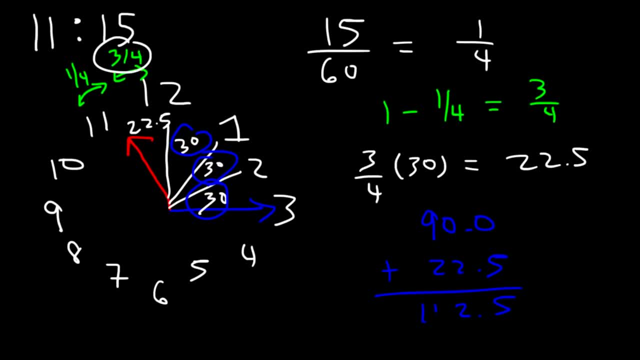 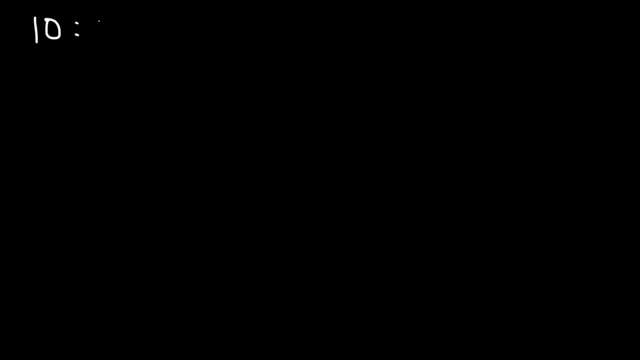 And so that's going to be 112.5.. So that is the angle between the hour hand and the minute hand. It's 112.5.. So here's the last example: Find the shortest angle for the time of 1025.. 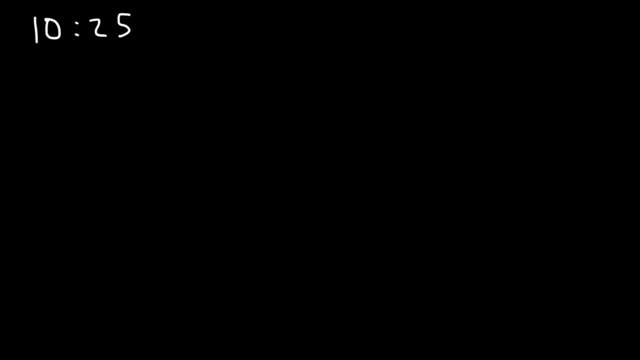 Find the shortest angle between the hour hand and the minute hand when the clock says 1025.. This is going to be 12,, 3,, 6, and 9.. So 25 corresponds to 5.. That's where the minute hand. 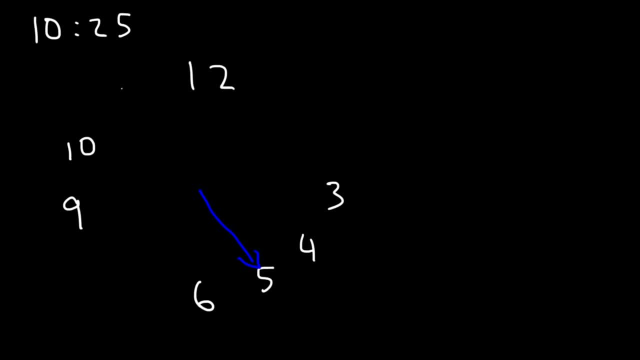 is going to be located Now. the hour hand is between 10 and 11.. So it's very close to the middle, but it's slightly closer to 10.. So there's the hour hand. Now let's find the fraction of 25. 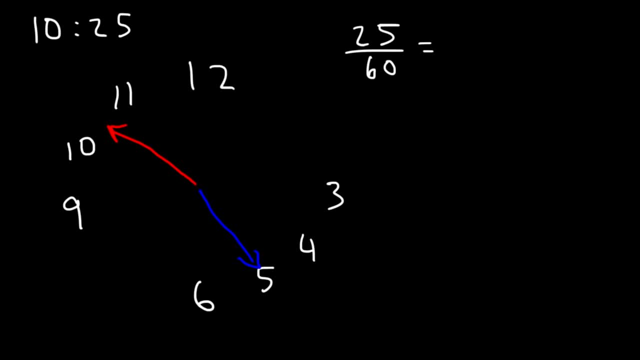 divided by 60. So 25 over 60.. 25 is 5 times 5.. 60 is 5 times 12.. So it's 5 over 12.. Therefore, between the hour hand and 10 is 5 twelfths of 30 degrees.